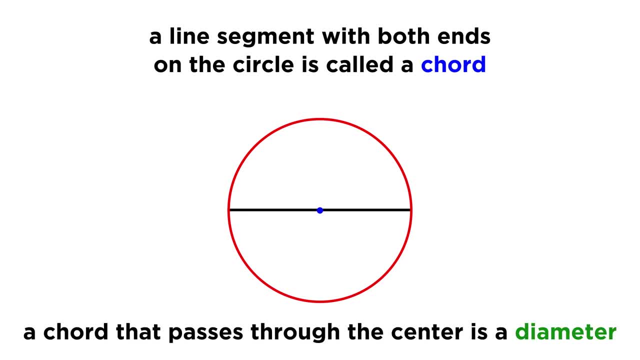 on the circle. A chord that passes through the center of the circle is called a radius. This is called a diameter, and we will note that the length of any diameter of a circle is always exactly twice the length of its radius. Lastly, any part of a circle defined by two endpoints is called an arc. 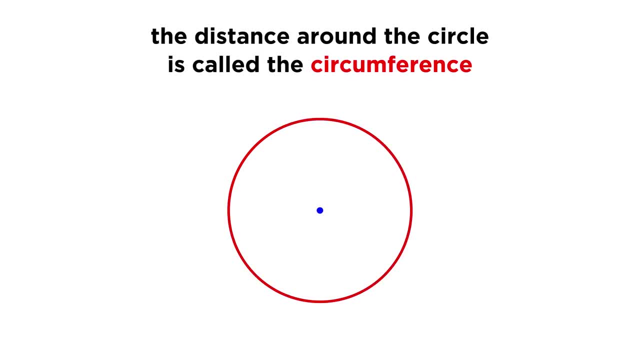 If this arc becomes the whole circle, which represents the distance around the circle or the perimeter of the circle, this is called the circumference. Just the way that the diameter and radius are always in the circle, the circle is called the circumference. When we put this in a two to one ratio, the circumference and the diameter also have a 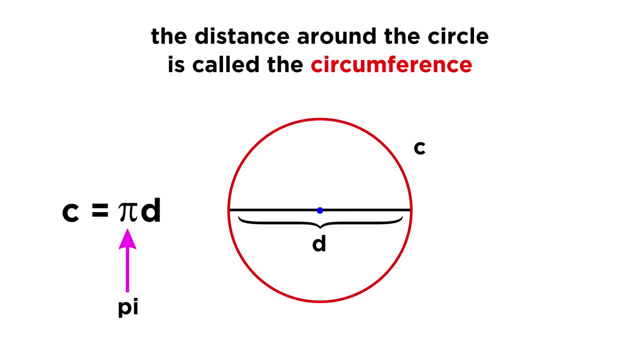 special ratio, and that ratio is represented by the number pi. This is an irrational number which, as we discussed before, is a number that can't be expressed as the ratio of two integers. This means that it has a decimal representation with digits that go on forever without any. 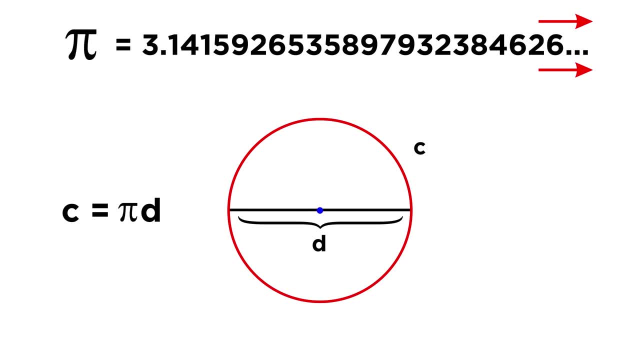 kind of repeating pattern, If you want to make sure that you're not boggling when you think about it. for our meager purposes, we can just estimate pi as being three point one four, as that will give us values that are precise enough to be meaningful. 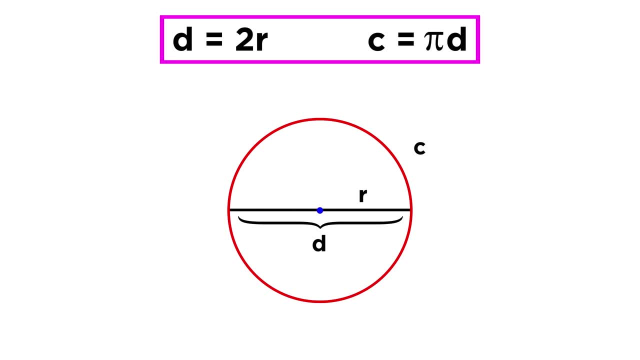 So the equations we need to know are as follows: D equals two R and C equals pi D. or, in terms of R, C equals two pi R, since one D is two Rs. Knowing this, if we are given any of these values, we can simply use the equation that. we just used to calculate the value of pi D. So the equation that we need to know is this: D equals two R and C equals pi D. Or, in terms of R, C equals two pi R, since one D is two R's. 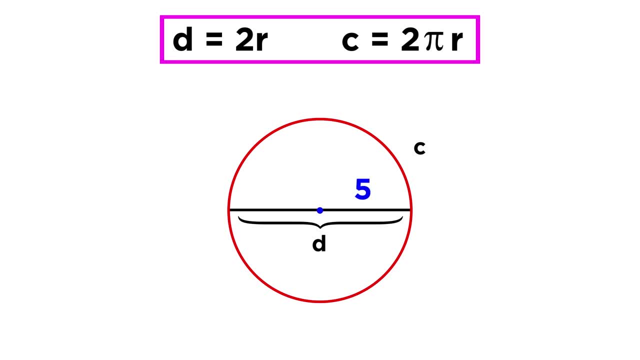 If we are given any of these values for a circle, we can find the others. For example, if the radius is five, what is the circumference? Well, we can double the radius to get a diameter of ten, and then multiply by pi to get a circumference. 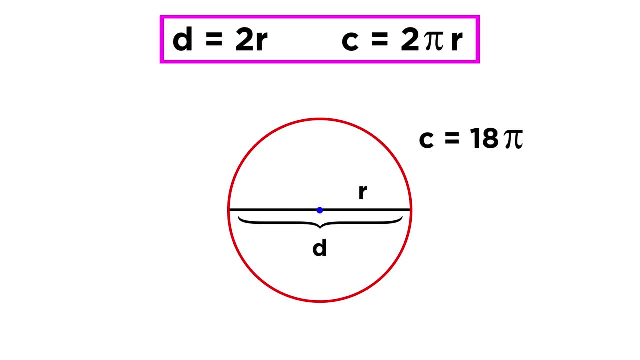 of ten pi Going backwards. if we have a circumference of eighteen pi, we can find a diameter of eighteen and a radius of nine. If we draw several radii on one circle, we will demarcate several sectors of that circle. A sector is a part of a circle enclosed by two radii and the arc that connects them.